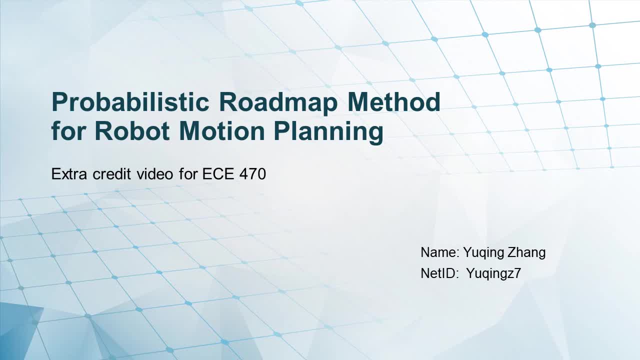 Hello everyone. today I'm going to introduce the PRM method for robot motion planning. Path planning is the basic for various tasks for robot and has always been a research hotspot. It is an important method for robot to avoid obstacles in the configuration space And in 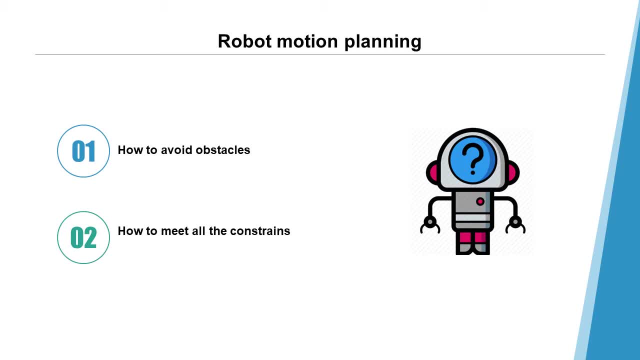 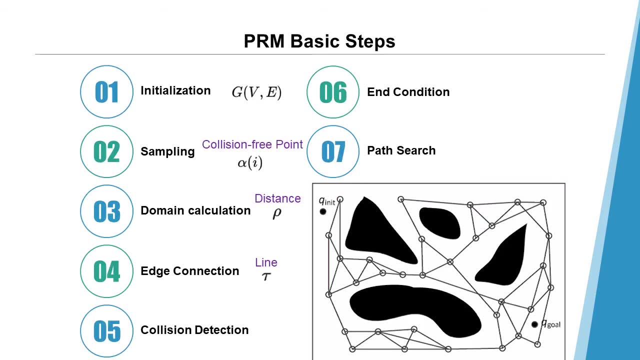 this video I'm going to focus on one type of sampling-based path planning algorithm, the PRM method. This method can be separated into the following steps. First, initialization: We set up an undirected graph where the vertex set V represents for all. 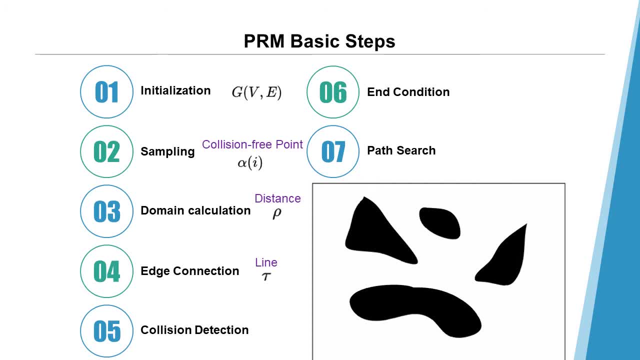 the collision-free configurations and the connection set E represents for all the collision-free paths. The initial state is empty. Second sampling: We sample a collision-free point in the configuration space and add it to set V. Three domain calculation: We define a distance rho for all the vertex in set V. 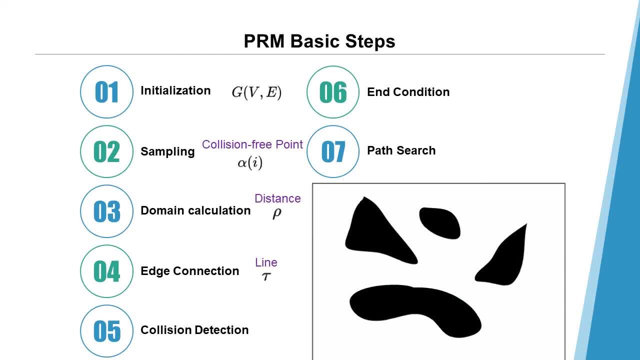 If its distance between alpha i is less than rho, we call it the neighborhood point of alpha i. Four: edge connection: We connect alpha i with its neighborhood point and generate a line tau. And five: collision detection. If tau doesn't collide with the obstacles, add it to the connection set E. 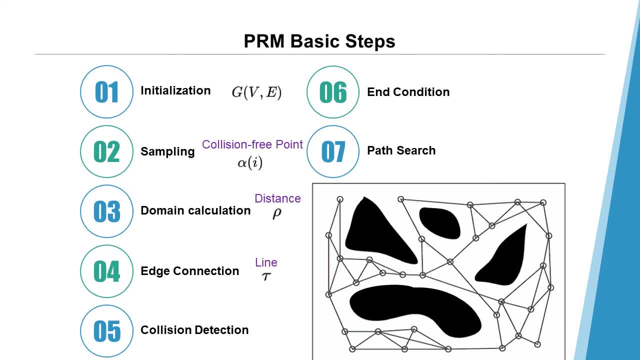 Six end condition: If all the sampling points have completed the above steps ends. Otherwise repeat step 2 to 5.. And the final step 7, if all the step above is finished. we use graph search algorithm in the undirected graph G to find if there exists a path from the 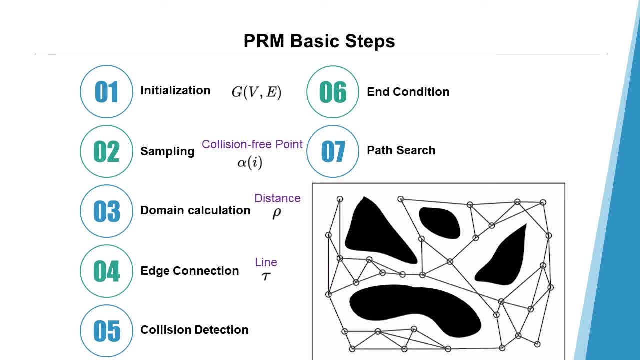 initial position to the destination. And if there exists one, then we find a path, And this page is the path to reach an object Like. this graph is a digital graph. If there is a path, access will be equal. So we correct this path, But there is no need for now to find the path At this point. z would put a math. 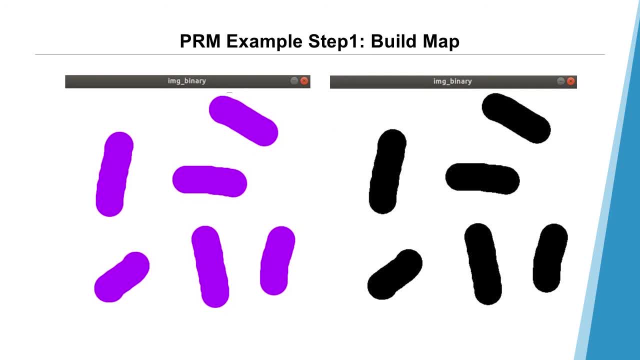 And the graph uniformizes. If there was no path, the path will fall off, but the path, non-linear or other way, would have to be carpeted into z how the algorithm works. Then let's take a look at an example. First, we draw a 500 times 500. 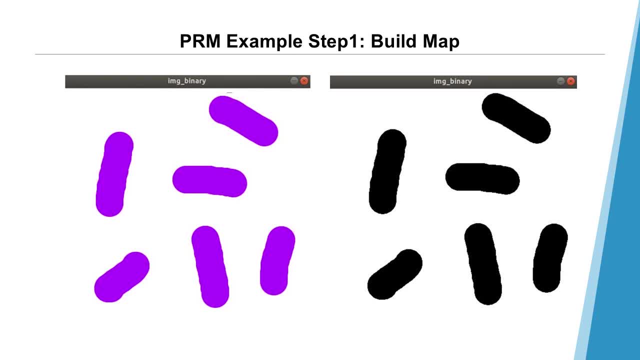 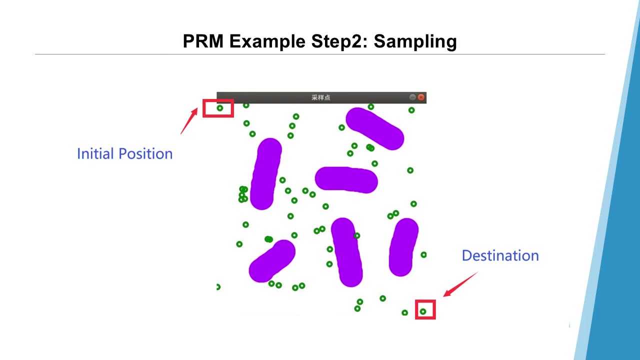 pixels image. The white area is the configuration space, while the colored areas are obstacles. Then we converted this image to a binary image for collision detection convenience And the second step is sampling. We randomly sample a specific number of collision-free points. 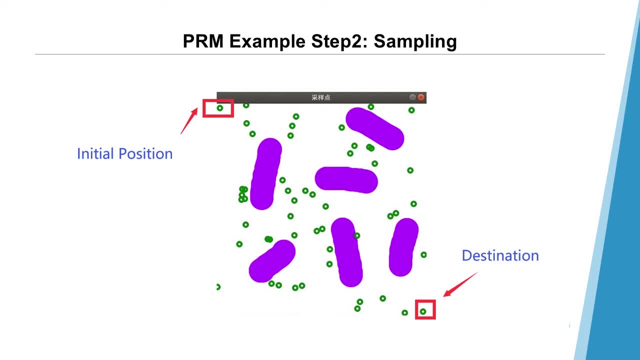 maybe 50 or 100, checking if all these points doesn't collide with obstacles. If some yes, then discard those collide points. In this image, the point on the top left corner is the initial position and the point on the right bottom corner is the destination. Step three: domain calculation. 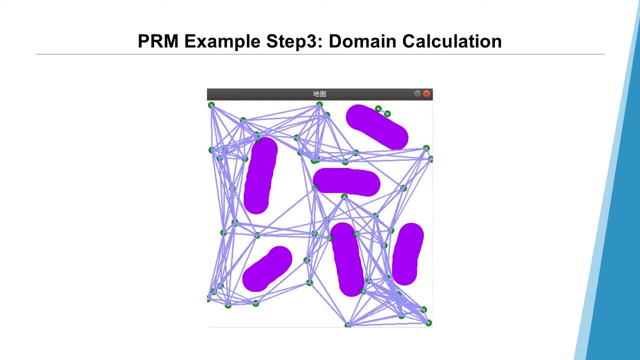 In this step, we connect lines between all these points and detect collision between lines and obstacles. However, we are not going to connect all the points, such as the initial position and destination. We only connect the points which distances are not too large, so we have to. 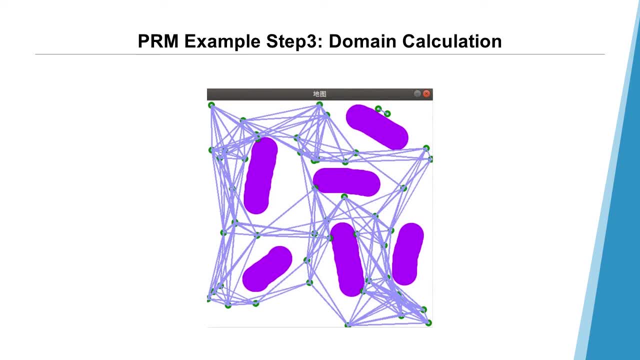 define the size of the domain. We will only consider these lines no larger than this domain size, maybe under 100 or 200.. After connecting and collision detection, we put all the collision-free lines into the connection set E. As we can see, since we have two points, we can only connect. 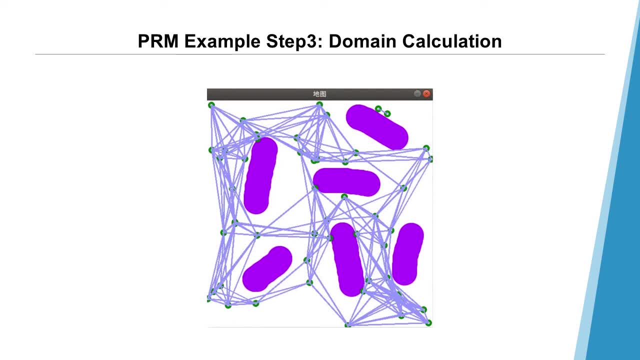 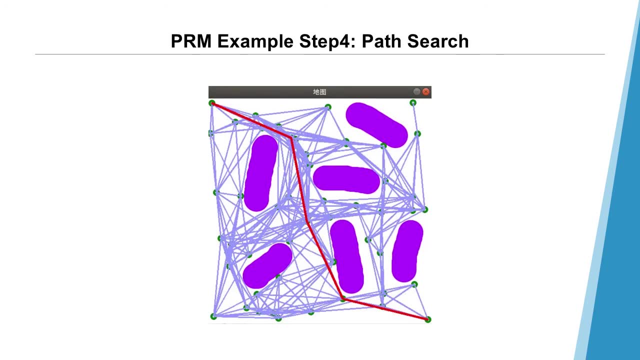 the domain and the collision constraints. There are two points on the top right corner- They have no connection with other points- And the last step, step four. we use a kind of graph search algorithm, such as the A-star method, to search the shortest path between the initial position and destination, And this path is the 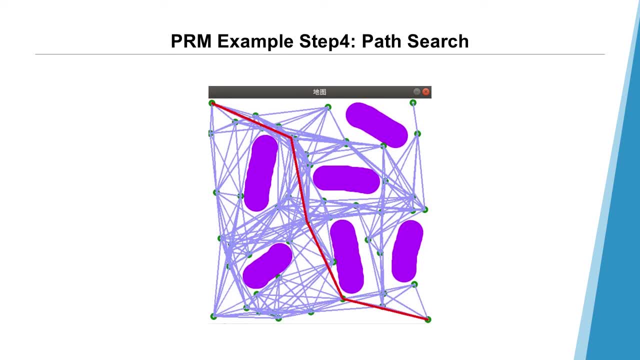 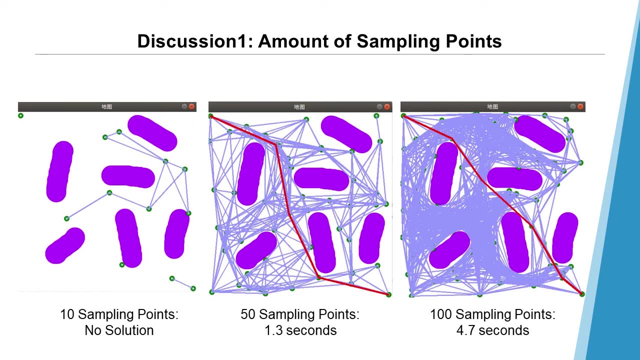 available shortest path, which is the solution to this problem. Then let's come to a conclusion on the PRM method. First, the amount of sampling points. It's clear that if we put more sampling points in this graph, we are more likely to get the shortest path, but relatively we'll spend more time searching this. 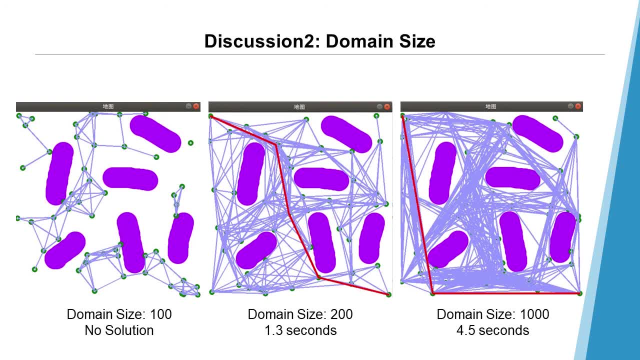 path. Second is the size of domain. It affects the generation of lines and collision detection. If the domain is too small, we may not find a possible line between points, And if there's no enough points, we may not find a possible line between points. So we can only search the shortest. 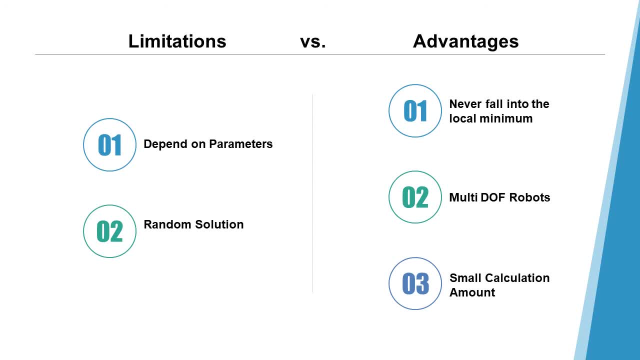 path of a solution. This method, proposed by Lidia in 1996, has three advantages. First, it overcomes the shortcomings that some previous path planning methods are easy to fall into the local minimum. And second, it can be applied to the path planning of multi-DOF robots. 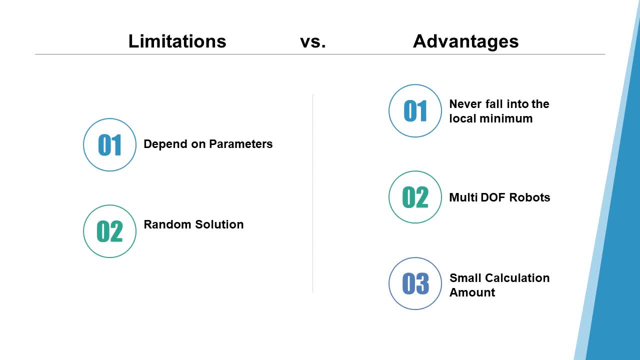 Third, small amount of calculation When the obstacles in the environment are more complicated- some previous path planning methods are more complicated, So we can only search the shortest path- will lead to a larger calculation, While the PRM can effectively solve the problem of path planning. 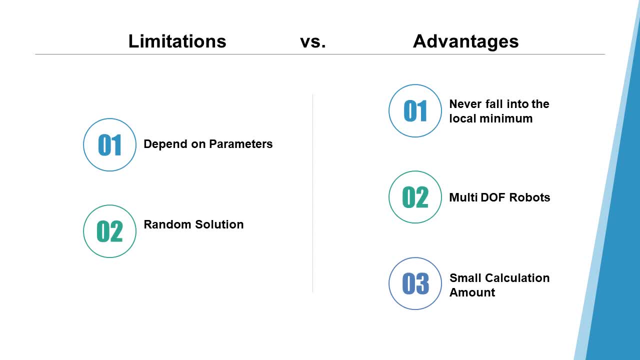 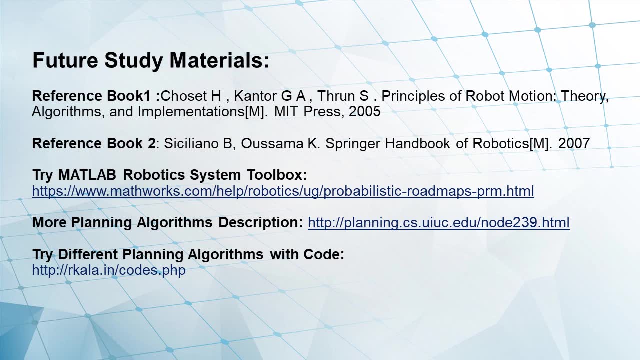 in high dimensional space and complex constraints. I have provided some materials for future studies. I have to say that it's quite fun to look through some of the traditional and advanced path planning algorithms, because I'm always amazed by the wisdom of these researchers and their technique in these. 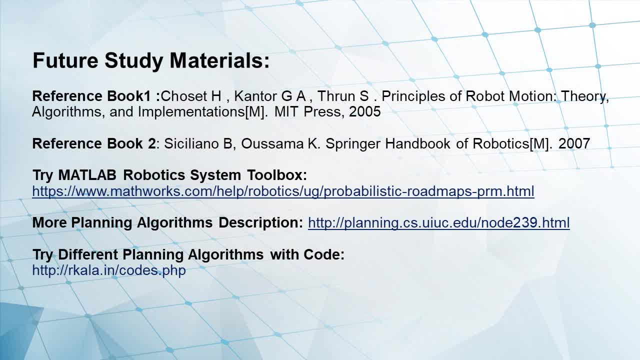 algorithms. And the third is the size of the domain, So we can only search the shortest path in the world. That's all for my video, Thank you. This is my references. 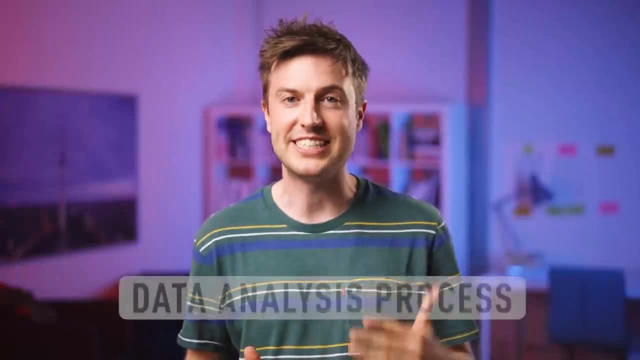 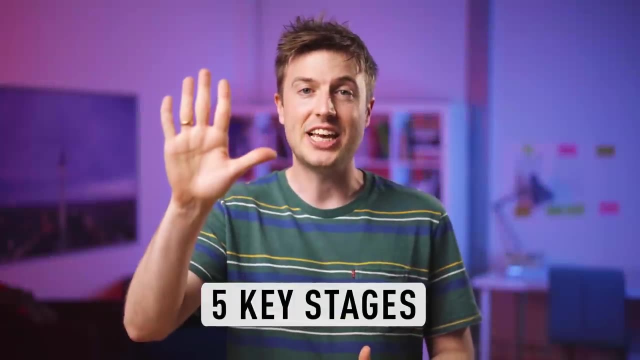 Hi, my name is Will and I'm going to give you a step-by-step guide to the data analysis process. Let's go. In this video, we're going to go through the five key stages of the data analysis process. We're going to give you an overview and. 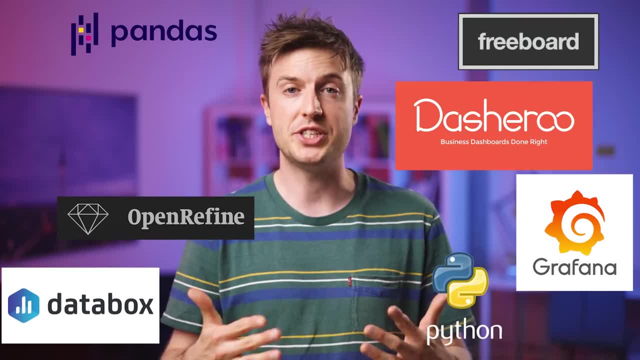 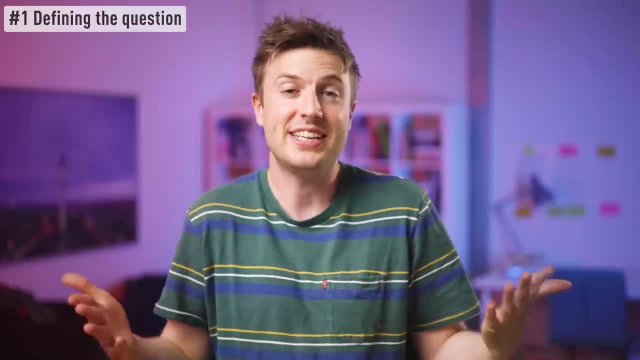 introduction to each of these stages, as well as looking at some of the tools you'll use to undertake these stages. So let's dive into step one: defining the question. The first step in your data analysis process, or any data analysis process, is to define your objective. In data analytics terms, this is called the. 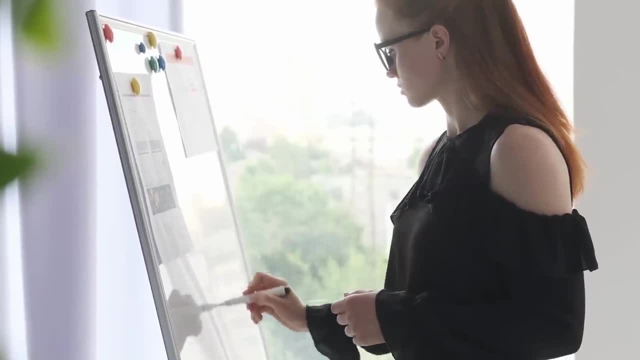 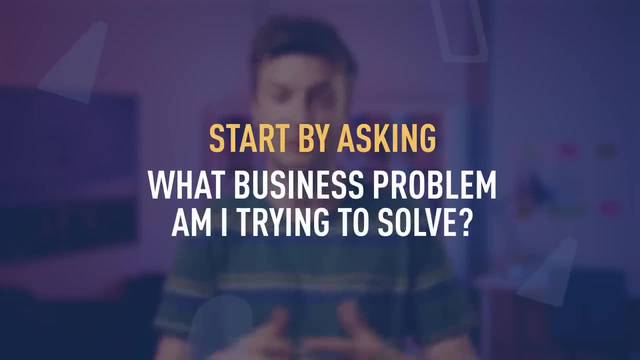 problem statement. Defining your objective means coming up with a hypothesis and figuring out how exactly to test it. You can start by asking: what business problem am I trying to solve Now? I know this might sound straightforward, but it can actually be trickier than it seems. For instance, your